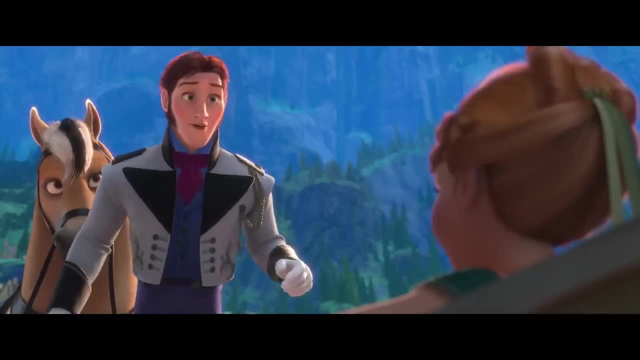 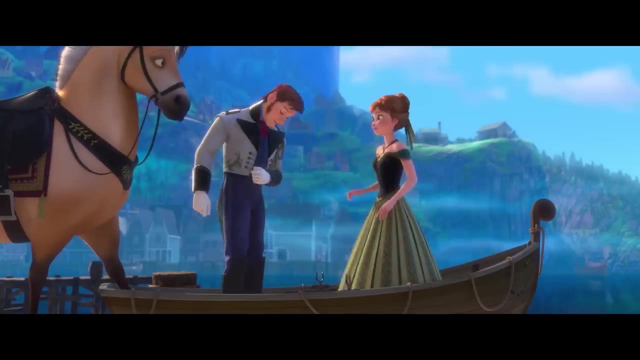 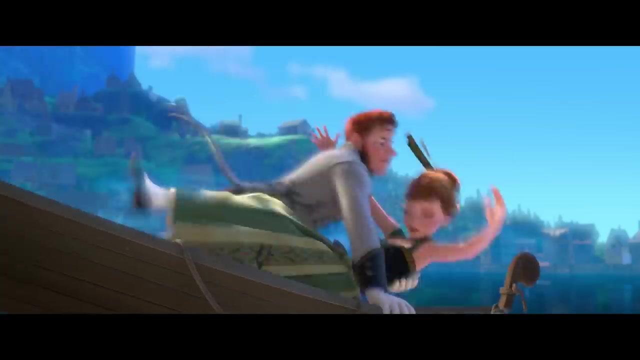 But I'm great actually. Oh, thank goodness. Oh uh. Prince Hans of the Southern Isles, Princess Anna of Arendelle, Princess Princess, My lady, Princess Whoa, whoa, whoa, whoa. 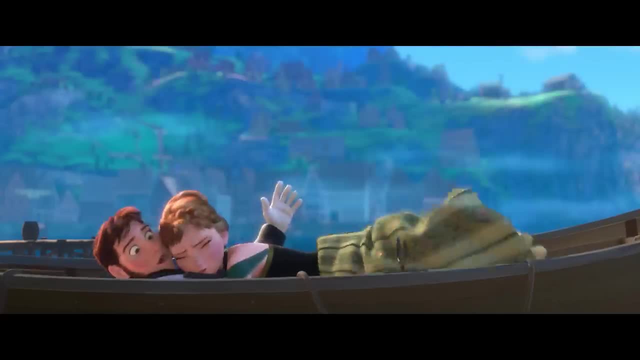 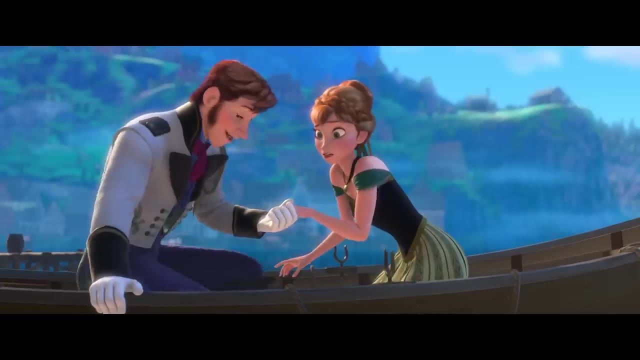 Oh, Um, Hi Again. Oh, Oh, boy, This is awkward, Not your awkward, but just because we're. I'm awkward. You're gorgeous. Wait what? I'd like to formally apologize for hitting the Princess of Arendelle with my horse. 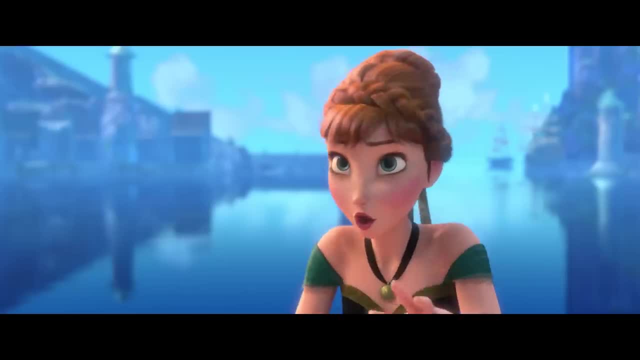 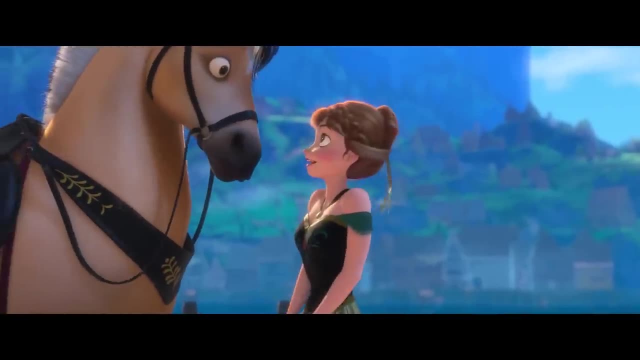 and for every moment after No, no, no, It's fine, I'm not that princess. I mean, if you'd hit my sister Elsa, it would be yeesh, Because you know, Hello, Hello, But lucky you. 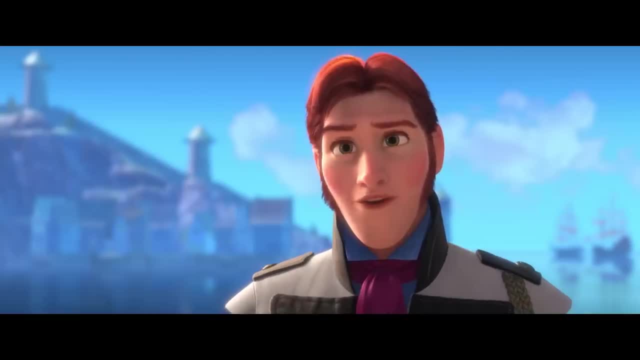 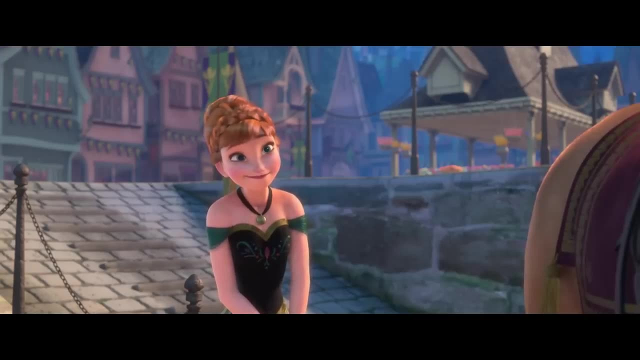 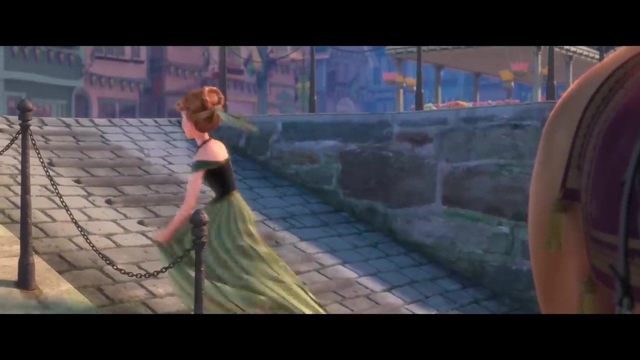 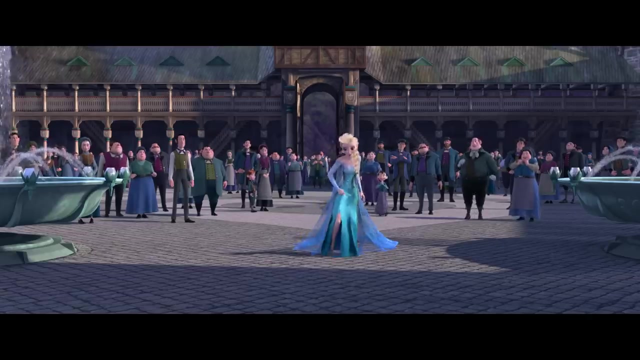 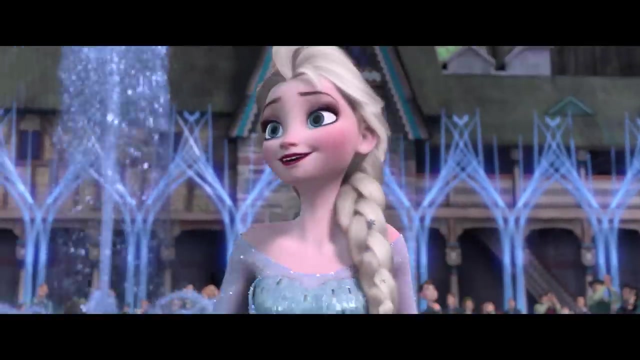 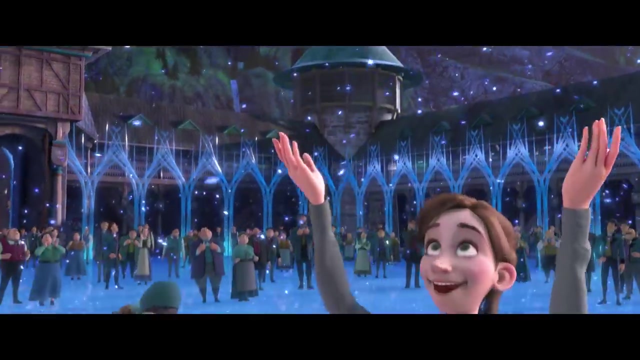 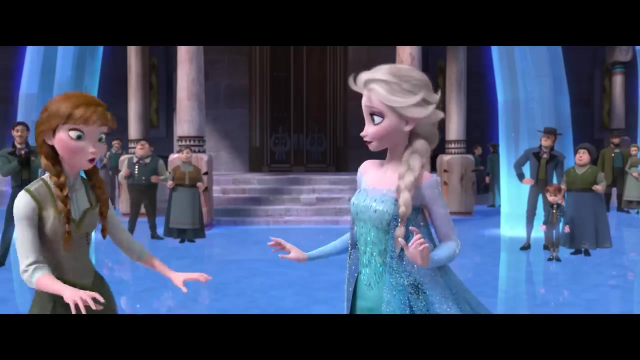 it's, it's just me, Just you. The bells, The coronation: I, I, I better go. I have to go, I better go. Bye, Are you ready? Yes, Whoo, Wow. I like the open gates. 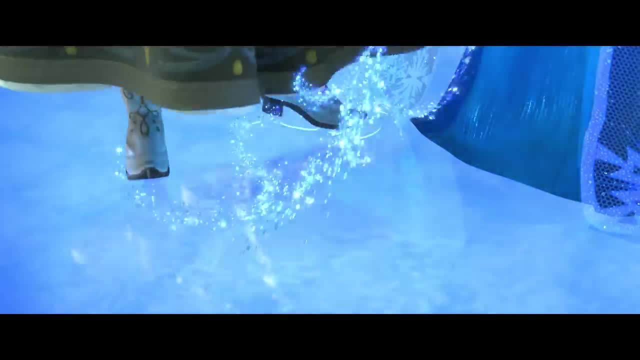 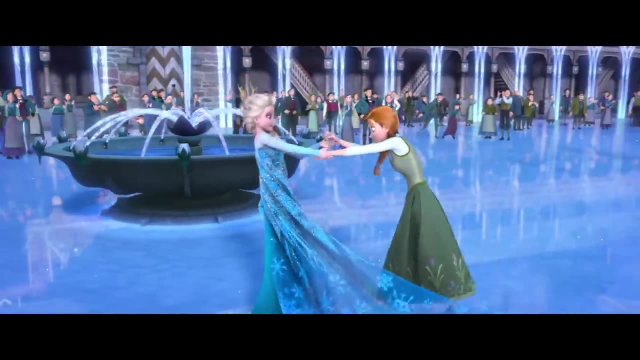 We are never closing them again. Oh, Elsa, they're beautiful, but you know I don't skate. Come on, you can do it. Look out reindeer coming through. I got it. I got it. I don't got it, I don't got it. 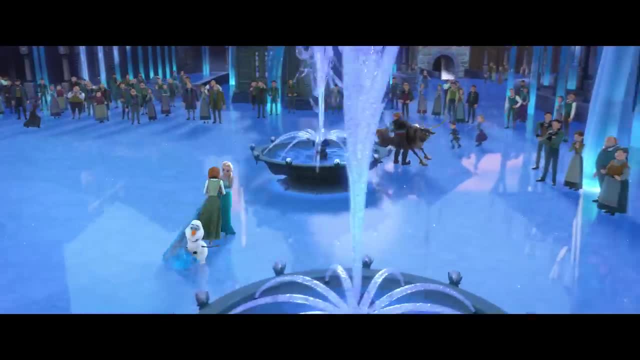 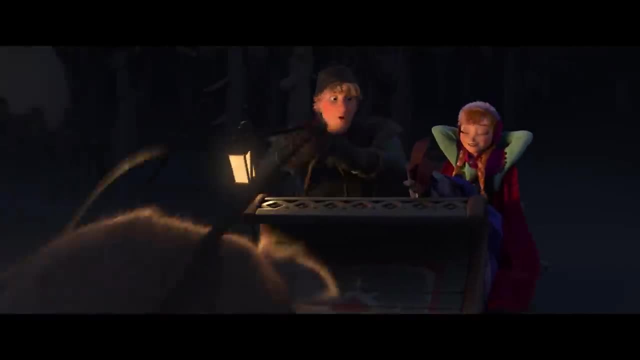 Hey guys, that's it. I love you. Glide and Hang on. we like to go fast, I like fast. Whoa, whoa, whoa, whoa, whoa, whoa. Get your feet down. 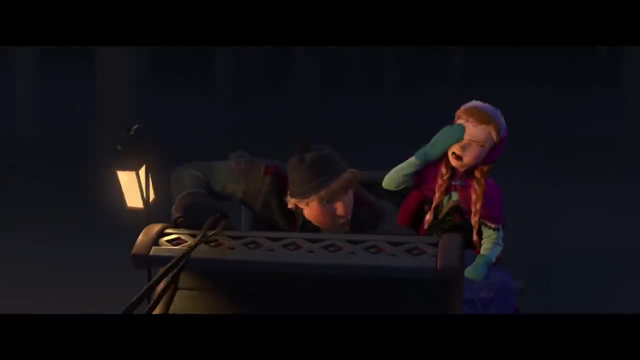 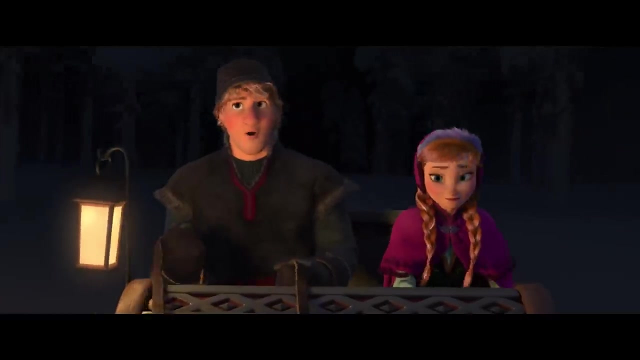 This is fresh lacquer. Seriously, were you raised in a barn? No, I was raised in a castle. So, uh, tell me, what made the queen go all ice crazy? Oh well, it was all my fault. I got engaged, but then she freaked out. 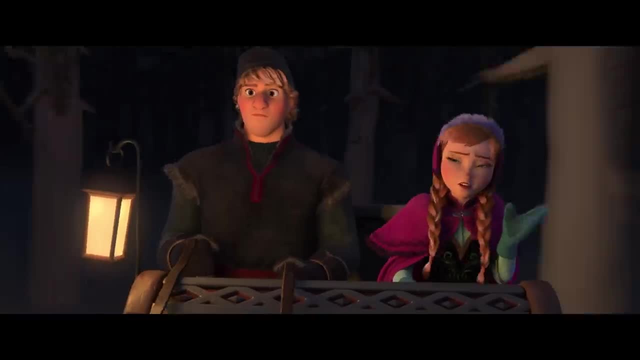 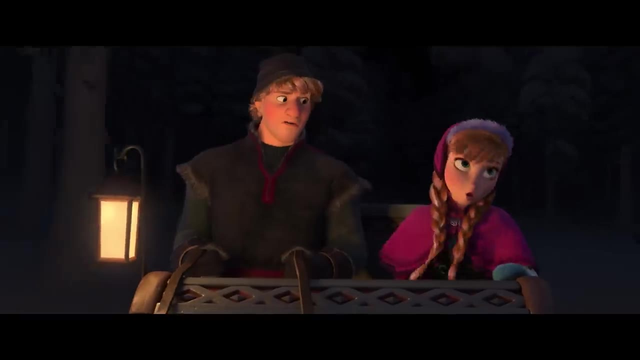 because I'd only just met him, you know that day, and she said she wouldn't bless the marriage. and Wait, you got engaged to someone you just met that day. Yeah, anyway, I got mad and so she got mad. 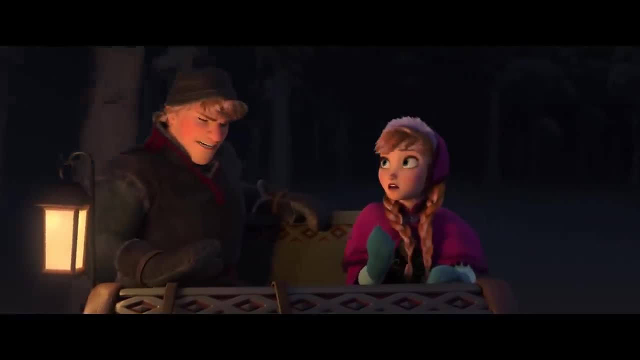 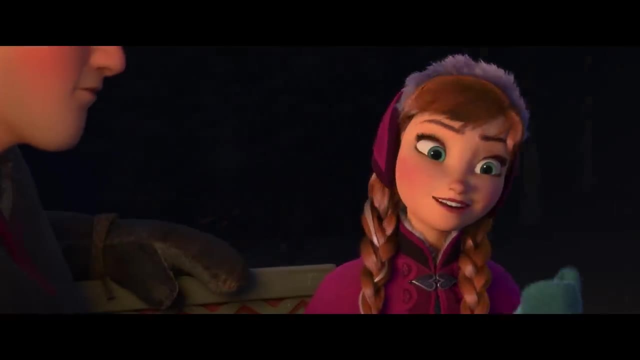 and then she tried to walk away and I grabbed her glove and Hang on. you mean to tell me you got engaged to someone you just met that day? Yes, pay attention, but the thing is she wore the gloves all the time. 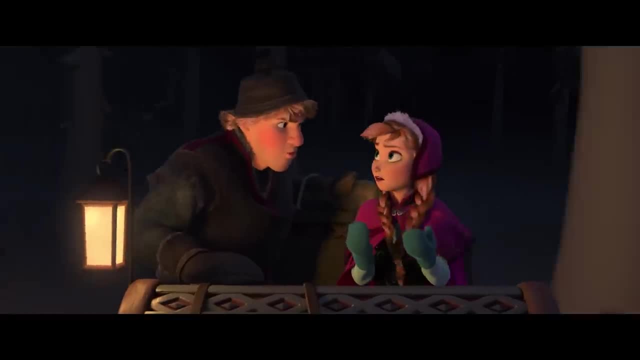 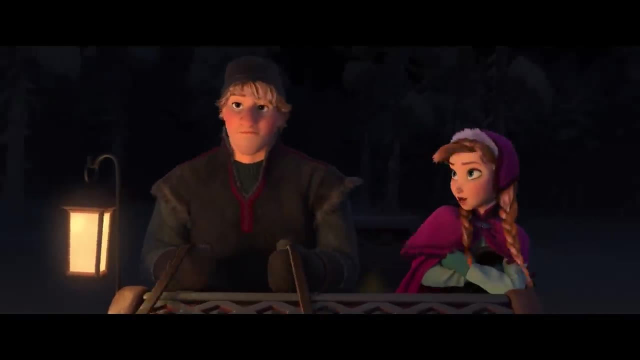 so I just thought maybe she has a thing about dirt. What Didn't your parents ever warn you about strangers? Yes, they did, But Hans is not a stranger. Oh yeah, What's his last name Of the Southern Isles? 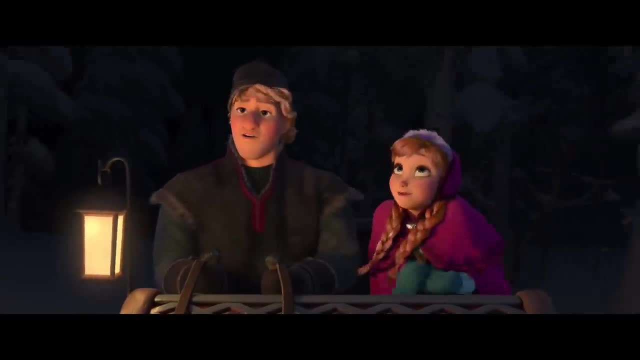 What's his favorite food? Sandwiches. Best friend's name, Probably John. Eye color: Dreamy Foot size- Foot size doesn't matter. Have you had a meal with him yet? What if you hate the way he eats? What if you hate the way he picks his nose? 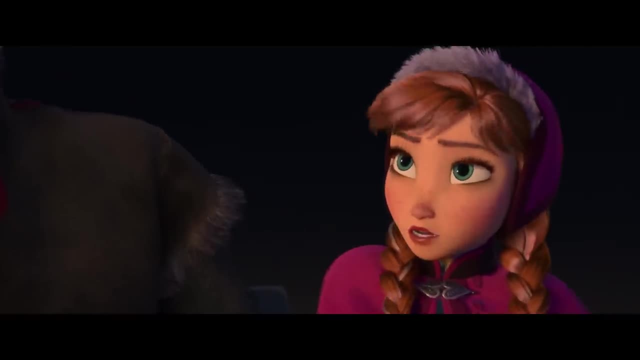 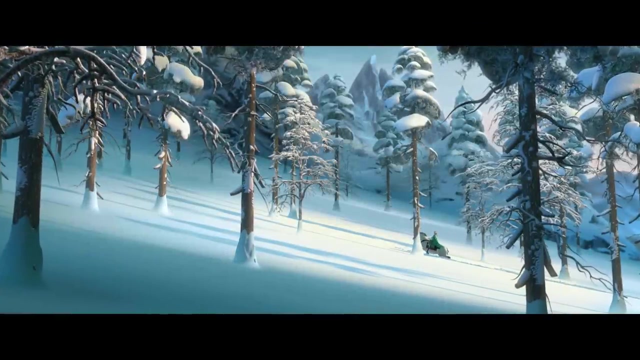 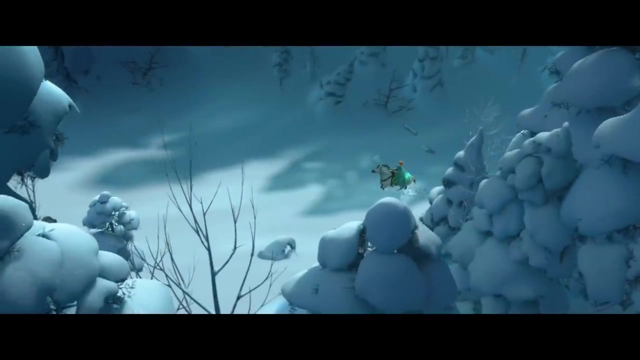 Picks his nose And eats it. Excuse me, sir, he is a prince. All men do it. Ew, Ew, Elsa, Elsa, Elsa. it's me, Anna, your sister, who didn't mean to make you freeze the summer. 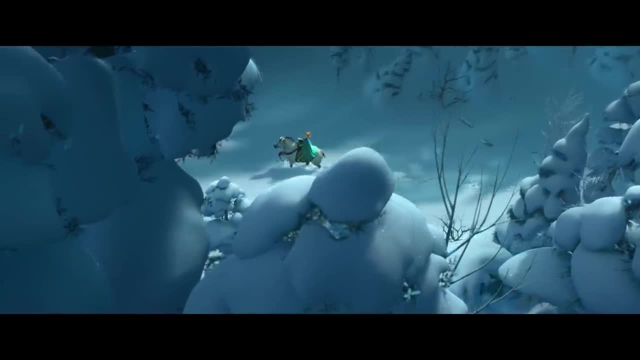 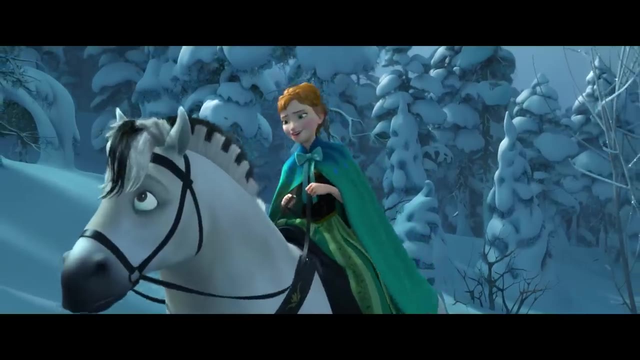 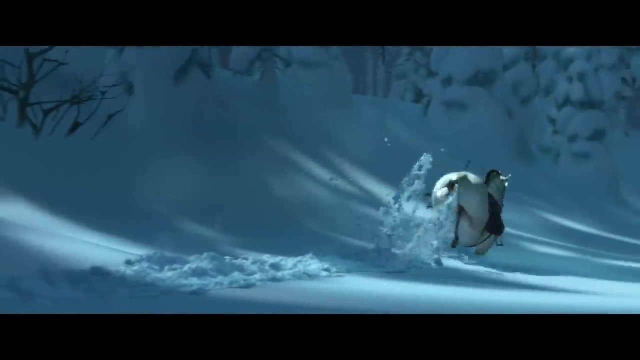 I'm sorry, it's all my fault. Of course, none of it would have happened if she just told me her secret. She's a stinker. Whoa, Whoa, Whoa, Whoa. Oh, no, no, no, no, come back. 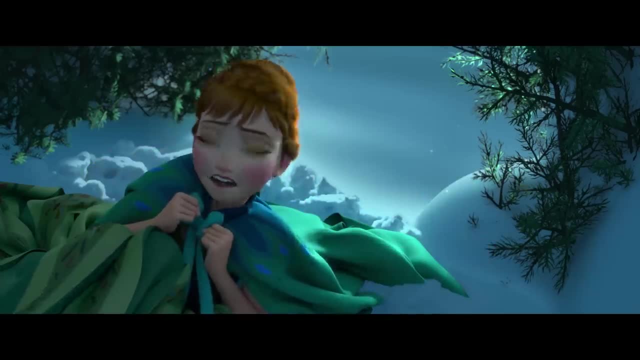 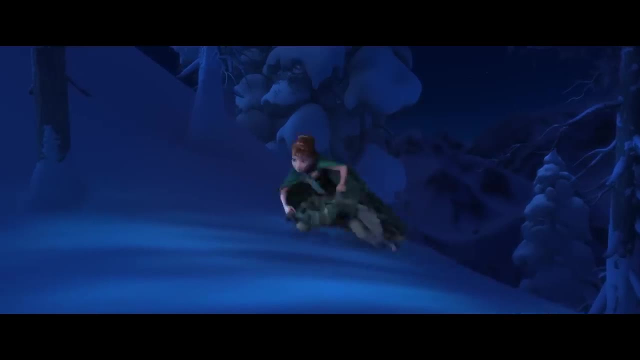 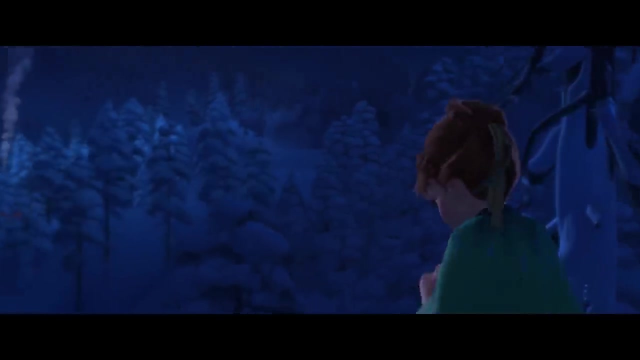 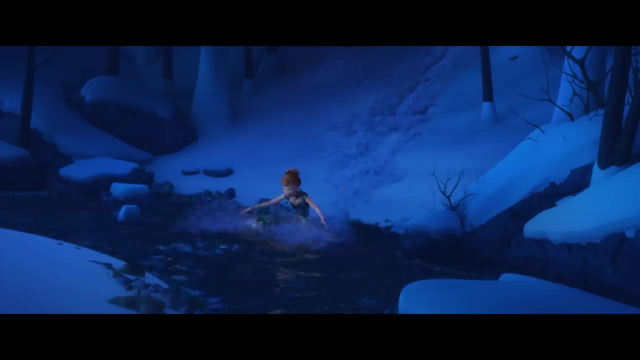 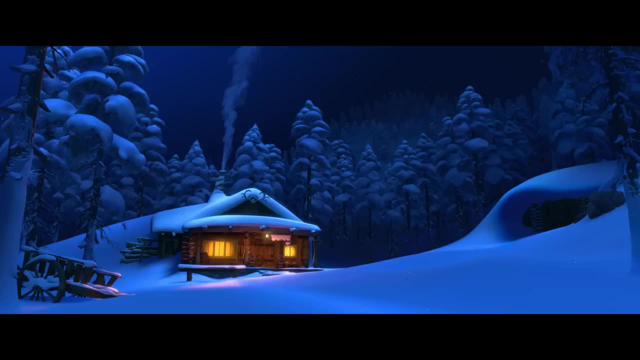 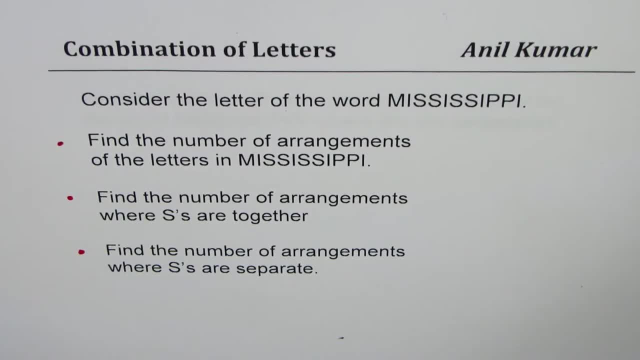 I'm Anil Kumar. We'll discuss combination of letters for the word Mississippi in this particular video. So we'll look into three types of questions. The first one here is: find the number of arrangements of the letters in Mississippi Right, that's straightforward.